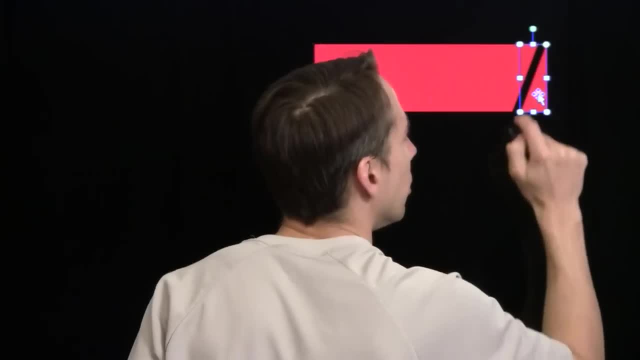 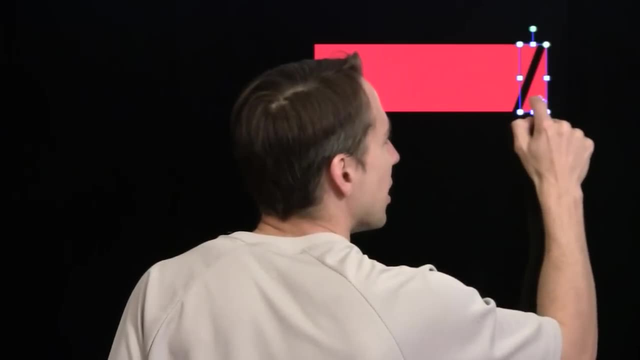 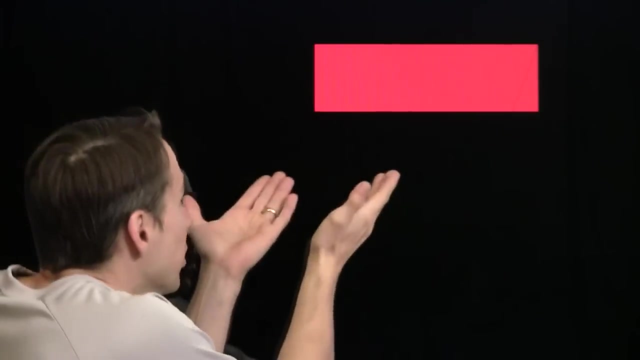 So I'm going to grab this triangle and slide it over here. This angle plus this angle in here, those two add up to 180 degrees. So that means we can slide this triangle in here and these go together and make a nice straight line there. So we do, We have a rectangle. 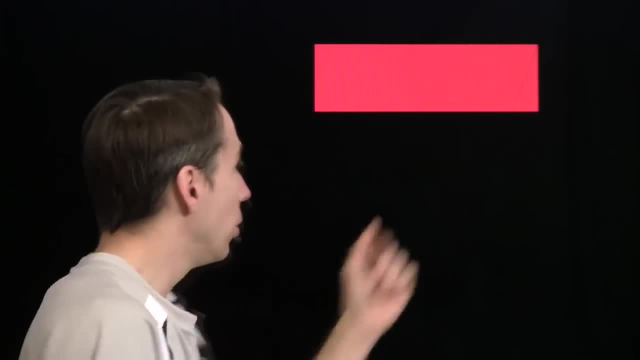 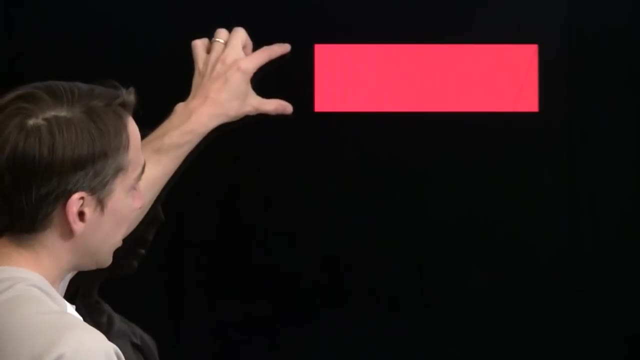 You can see that from the angles. now, This is a right triangle, so that's a right angle. That means this is a right angle as well. These two sides, the top and the bottom, are parallel, so these two angles, right here they have to add up to 180 degrees. This one's. 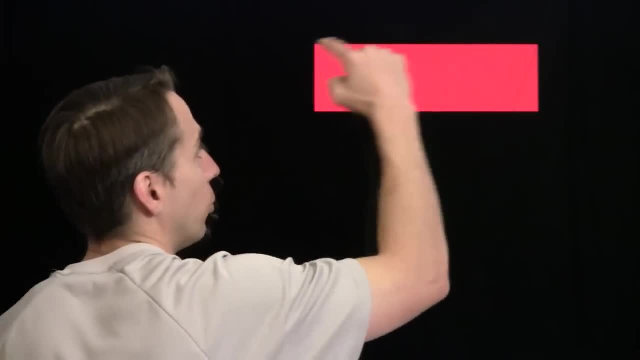 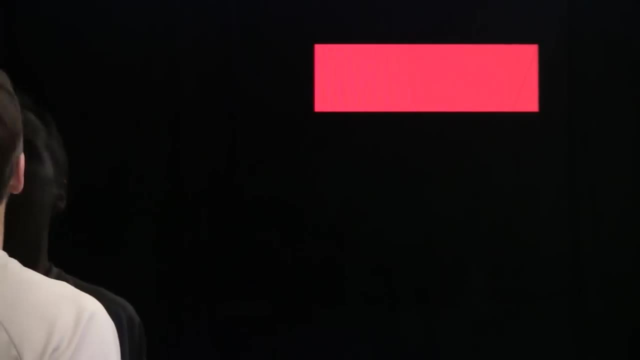 already 90, so this one has to be 90 as well. We have ourselves a rectangle and we know how to find the area of a rectangle. That's awesome, Harvey, right there. All right, We know how to find the area of a rectangle. It's just the base times, the height, It's. 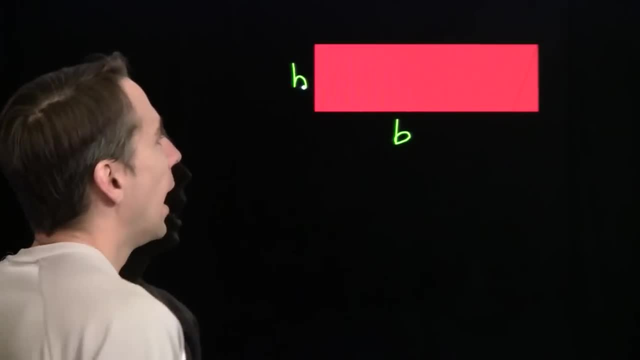 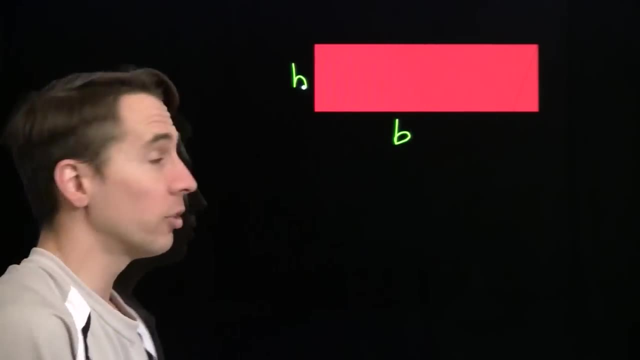 the product of the two dimensions And when we move these pieces around, we're not changing the area, The area of the parallelogram, when we took the triangle from here over to there. so the area of the parallelogram is also the base times the height, And also this is a rectangle. 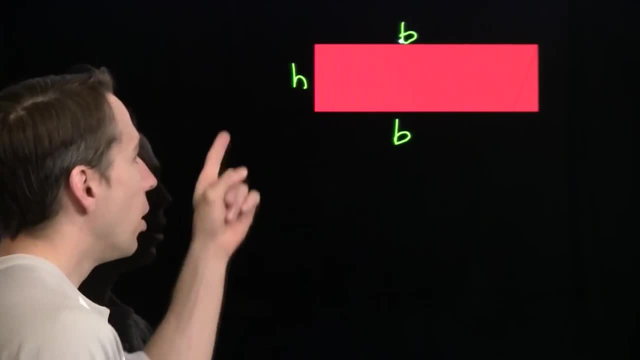 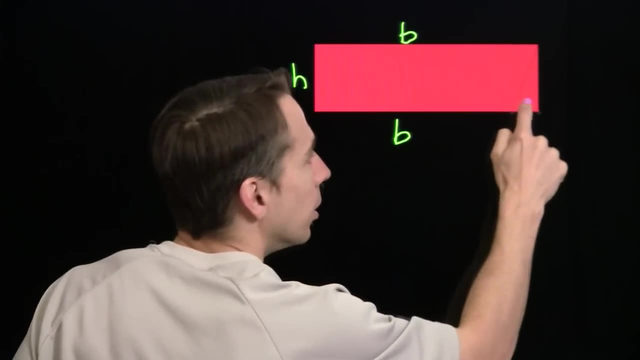 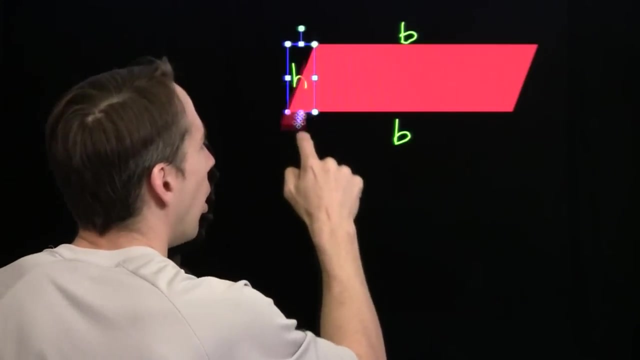 so the top here, that's a B as well. Now, when we're moving this piece back and forth, the area isn't the only thing that stays the same. The area stays the same, but so does the length of this bottom side. So we move this from here over to there. All we're doing. 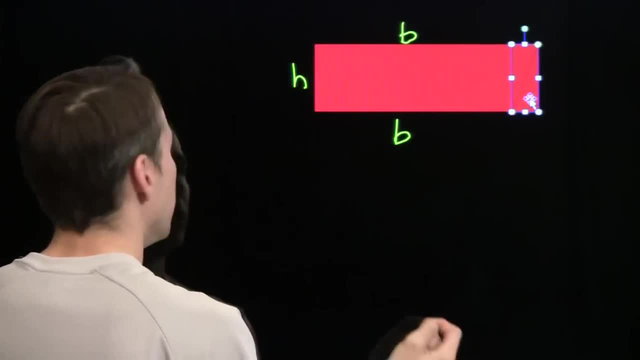 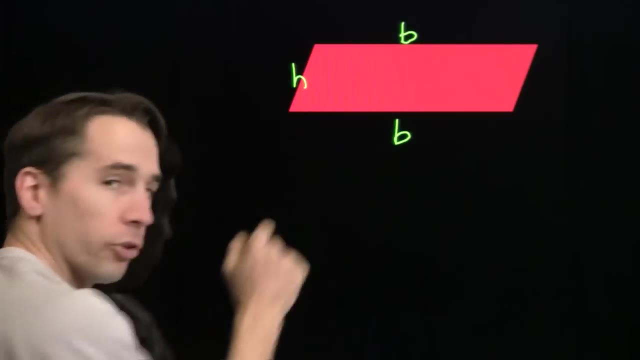 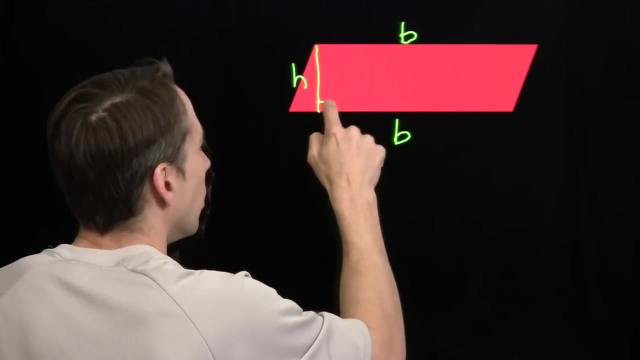 is moving a piece of the bottom from the left to the right And we can move it back. So this bottom of this parallelogram, its length is also B. I'm going to go ahead and put that height back in there. So now we also see that the 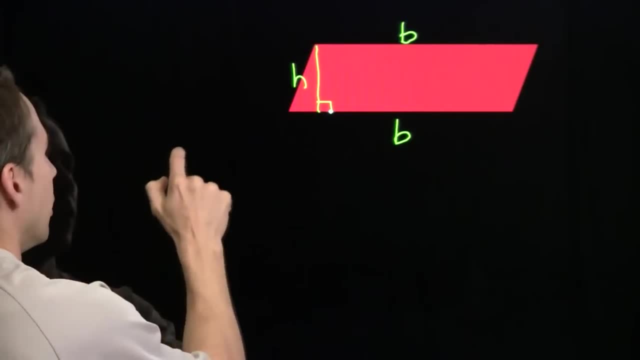 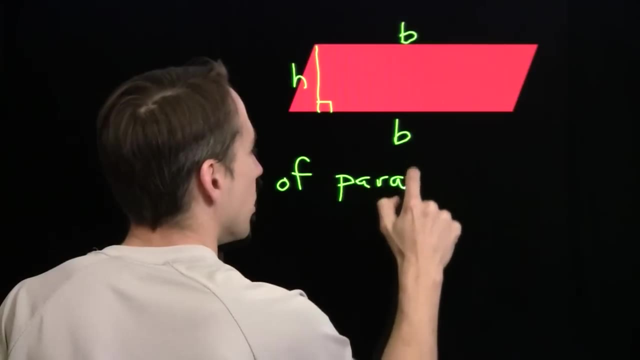 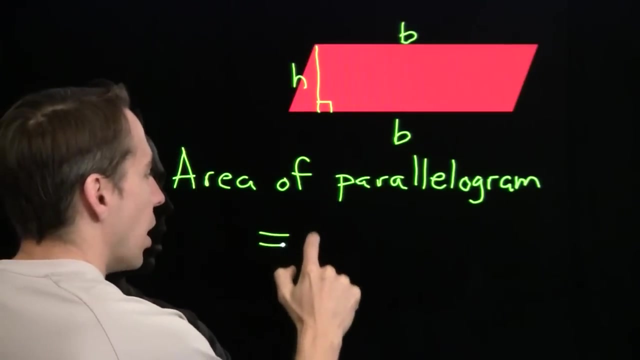 opposite sides of a parallelogram have the same length. All right, So we've got our area of a parallelogram now. It's just the base times, the height, And the height is the distance between these opposite sides, And these opposite sides are equal in length. What's that, Oh? 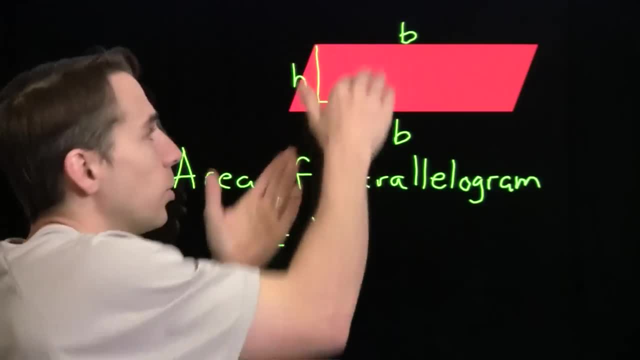 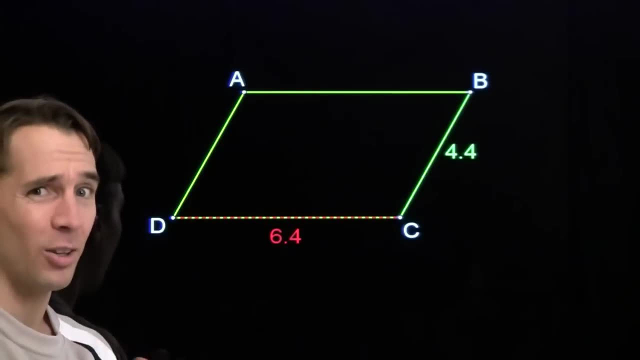 you don't buy my explanation of the opposite sides being equal in length. That's a little fishy. When you get into more advanced geometry you'll find a better way to prove it, But here's how I convinced myself. I thought it was a little fishy too, So I made this thing. 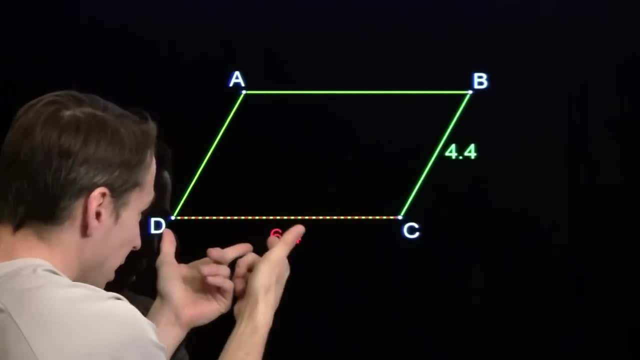 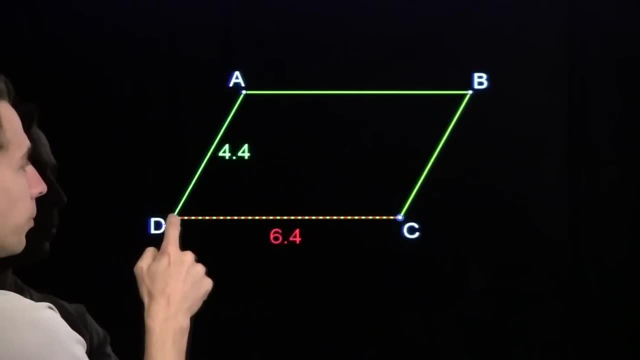 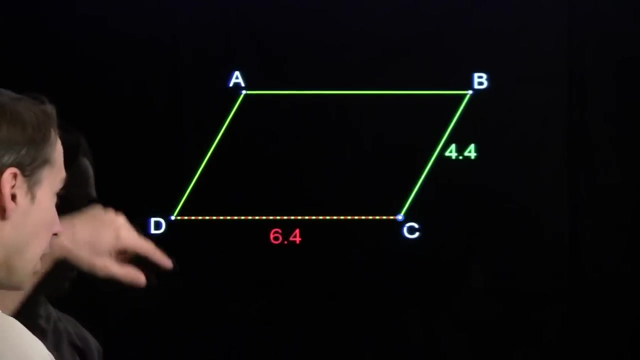 right here. It's a parallelogram. I've got the sides marked. This one's 6.4.. This one's 4.4 in length. Now watch this. I'll grab this. I can just slide this across. It stays 4.4 all the way. Same thing with the other side. 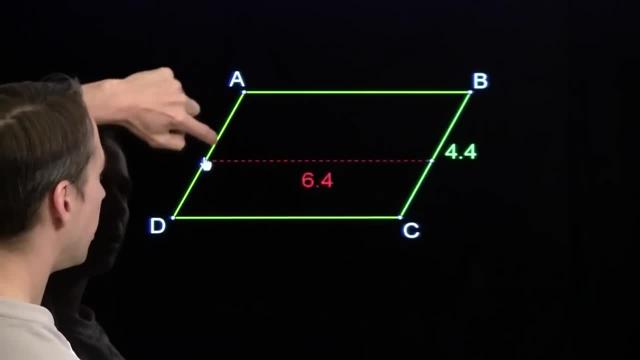 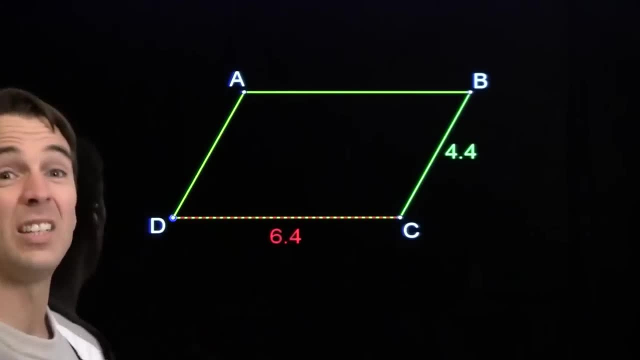 6.4 all the way. Now I know what you're thinking. You're thinking. I just made this little thing, put the numbers on there, and the numbers won't change, even if the lengths do change. But check this out. See, Numbers are changing. Lengths are changing, Numbers are changing. 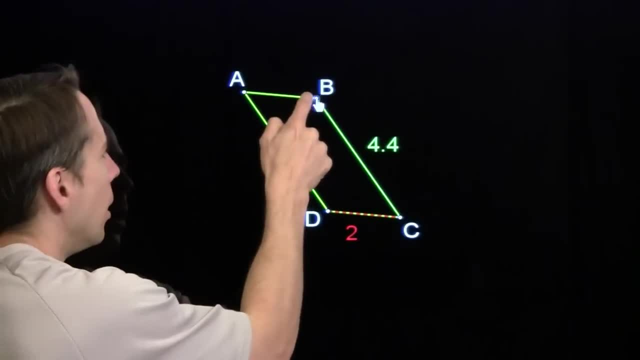 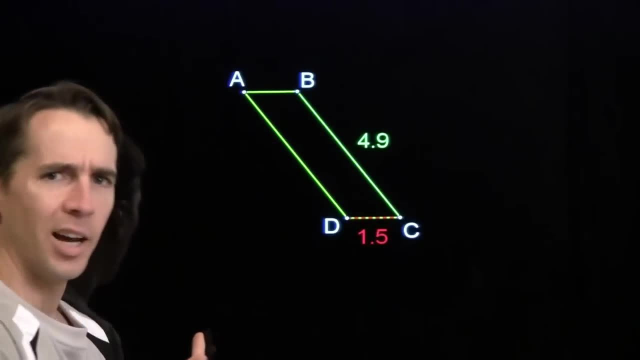 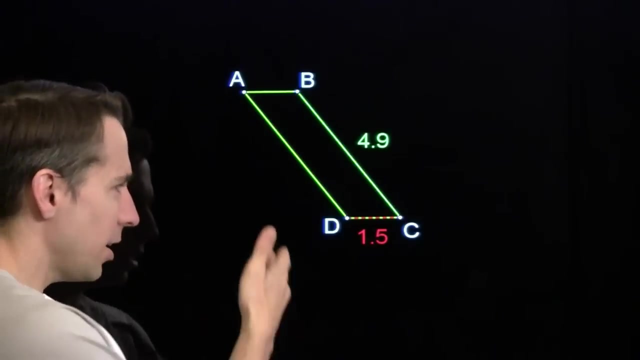 I'm not trying to trick you, At least not now. Hey, wait a second, I see something else that's pretty fishy. Check this out, Harvey. I don't quite buy your explanation of the area. Take a look at this. How are you going to chop? 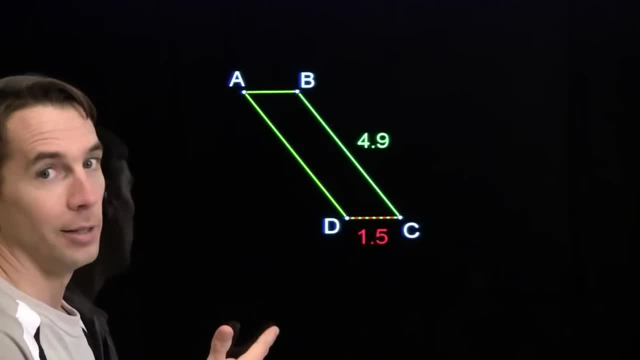 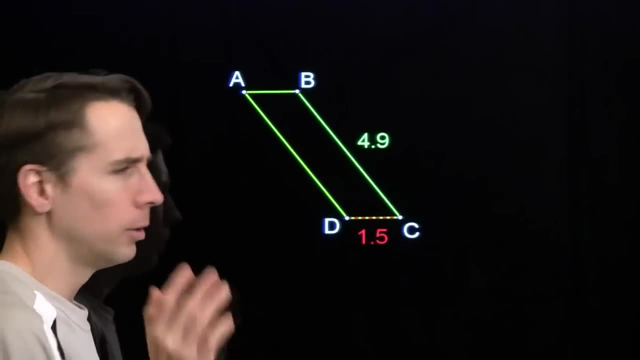 this up and make a rectangle. Got you now, don't I? I got him What? There's still a rectangle. Now you can't chop, this, slide one little piece and make a rectangle. Check this out. Check it out, Harvey. All right, Right, here, Right. 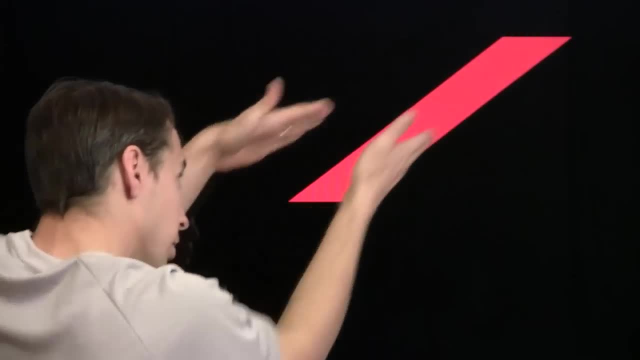 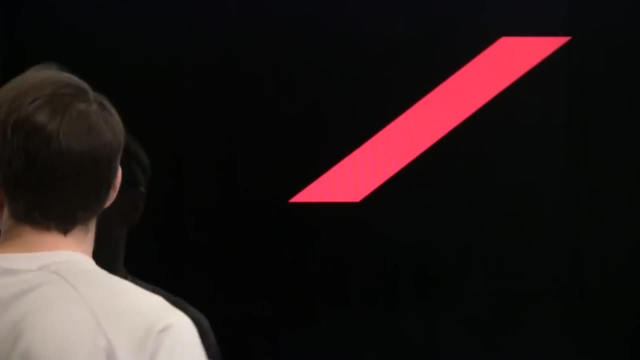 here. All right, Parallelogram, Still a parallelogram Side's parallel to this. These two are parallel And we want to show that this times the distance between these two opposite sides is the area, because we don't want to have a different formula for this parallelogram. as for this, 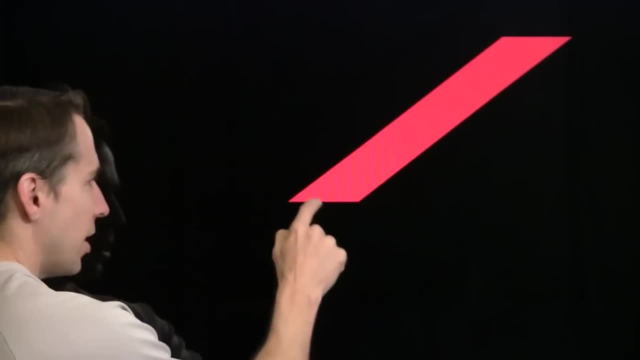 one. But you can't just chop this, slide it over and make a rectangle. Check this out, Harvey. Check this out. Yeah, you see it too, don't you? Yeah right, We're going to put this right up here. 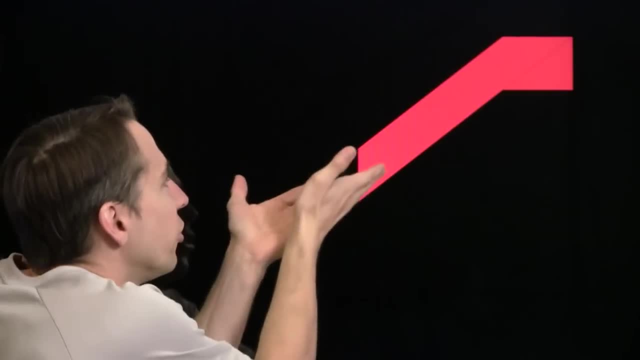 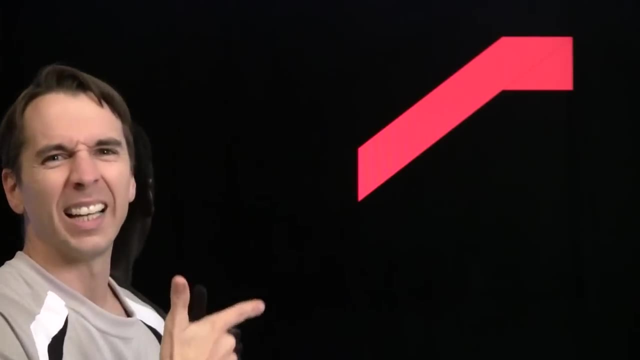 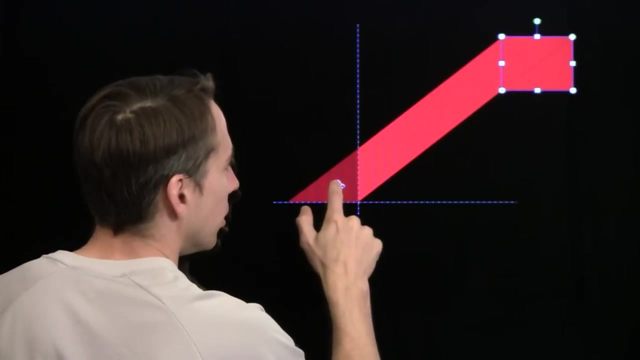 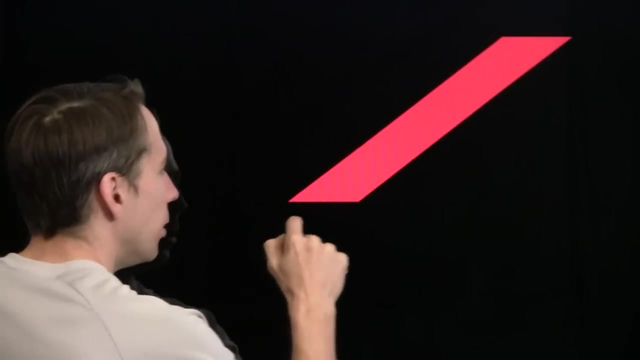 All right, Harvey. Where's the rectangle? This isn't a rectangle. One, two, three, four, five, six sides. Six sides, not four. Where's the rectangle? I got him What? Put it back, Okay. Where's the rectangle? Harvey, Outside the parallelogram? Okay, All right. Extend. 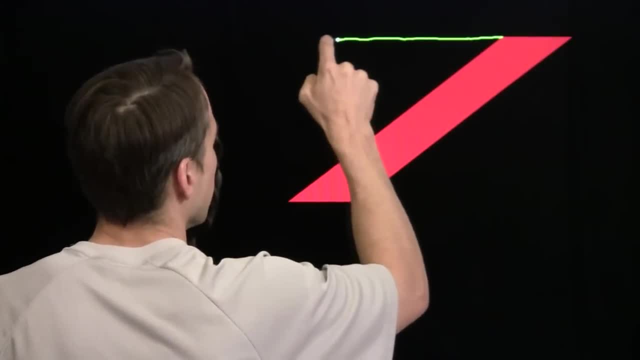 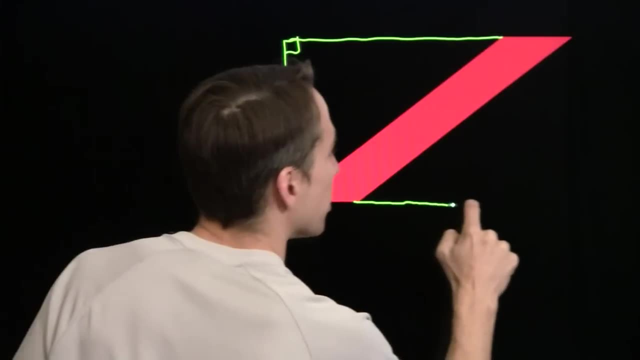 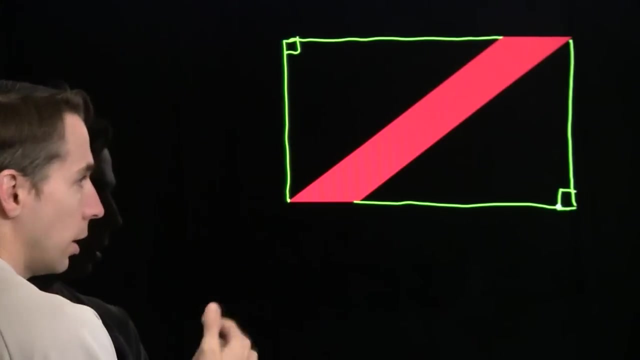 this. Extend the top and the bottom. All right, Extend this out, Okay, And come down here, Make a right angle there And do the same thing down on the bottom. All right, Now what Label the sides? Okay, We'll call that the height. still, It's the. 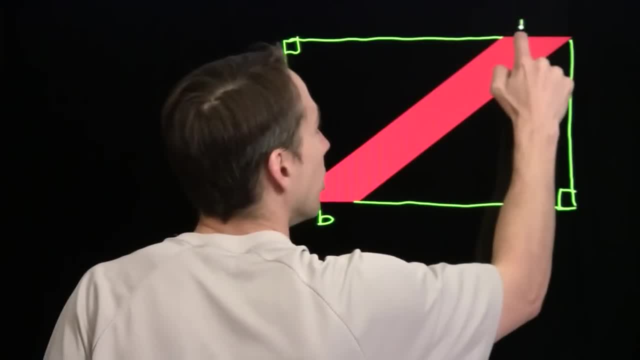 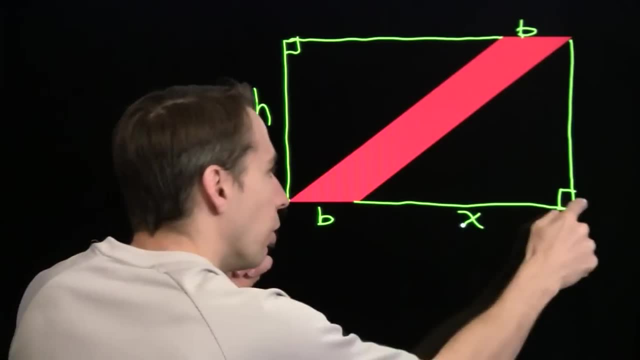 distance between the opposite sides, And we'll call this b and b, And we'll call that x. And well, this is a rectangle. This is a rectangle, So this is b plus x. That means this up here has to be b plus x. 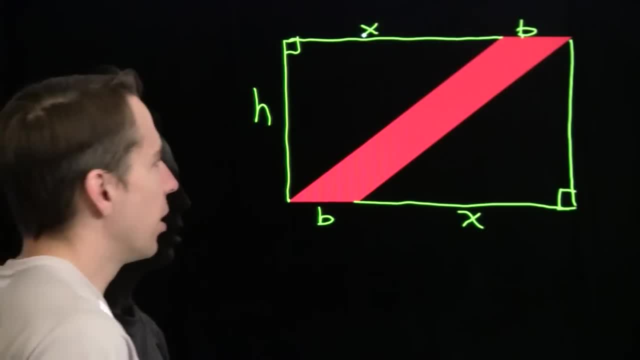 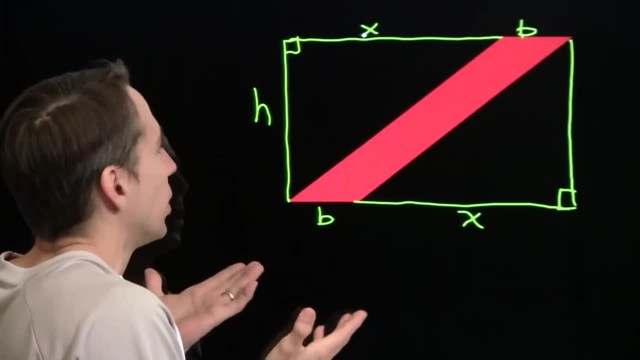 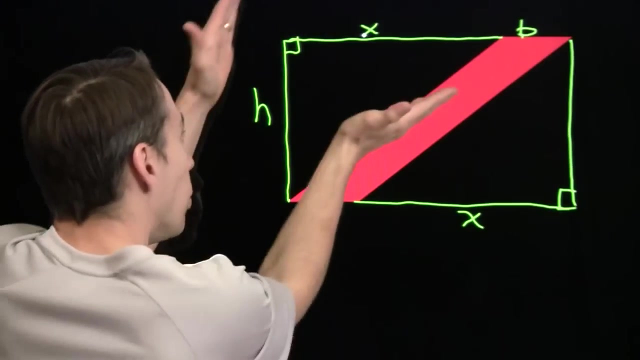 Now, what do we do? Find the area of the parallelogram. Oh yeah, This is that cool strategy we've used a bunch of times with area. We express the area of the parallelogram in terms of pieces we can handle. We can handle the rectangle, We can handle the right triangles, All right. 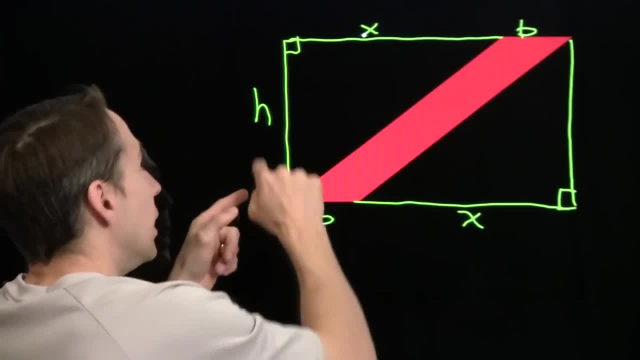 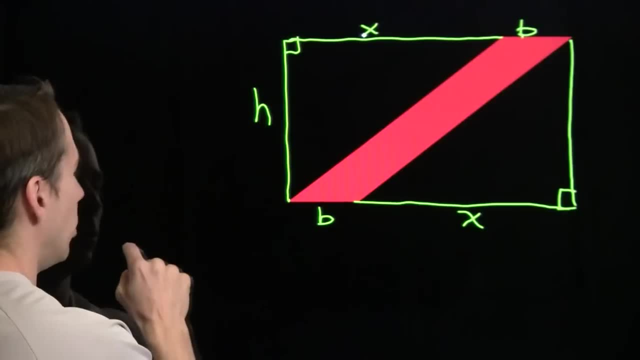 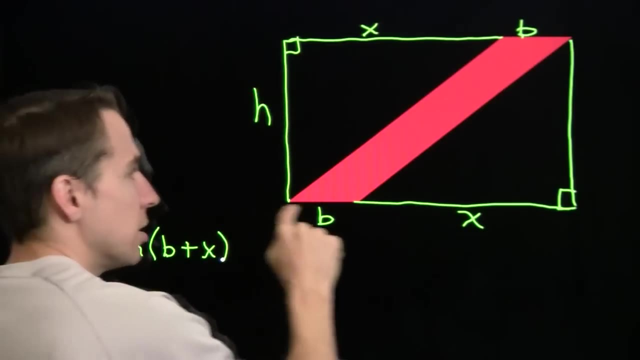 Let's do that. So the area of the parallelogram is the area of the rectangle, minus the areas of the triangles. So the area of the rectangle, well, that's just h times b plus x, This dimension times this dimension, And then we have to subtract off the areas of the two right triangles. 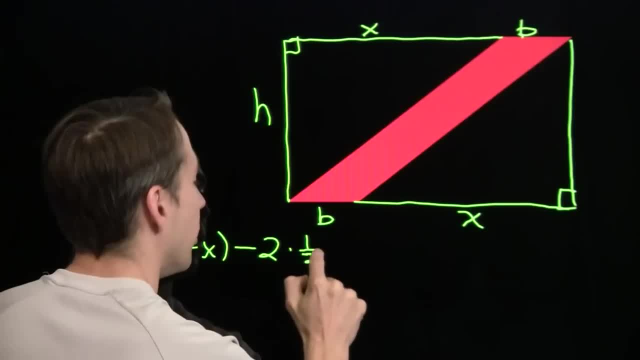 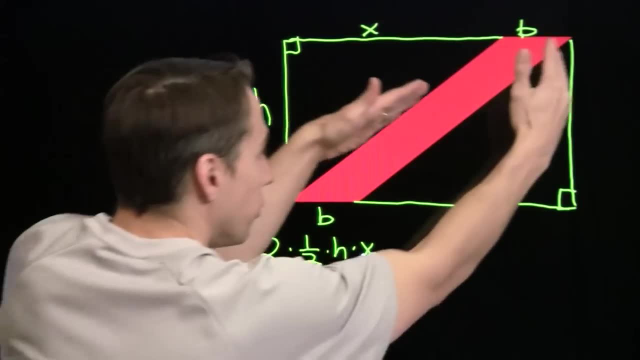 The area of the right triangle is just 1 half times the product of the legs, times h, times x, And we have to multiply by 2 because we have two of these right triangles. So to figure this out, well, we'll go ahead and expand this product. 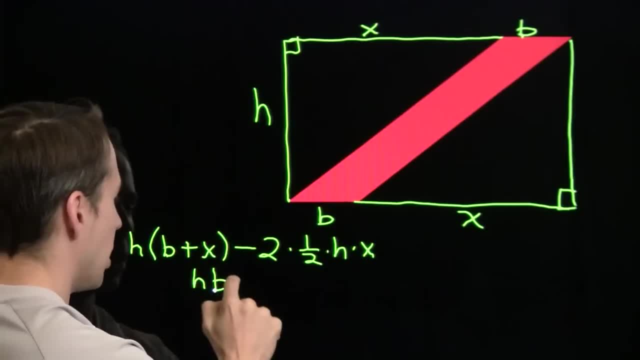 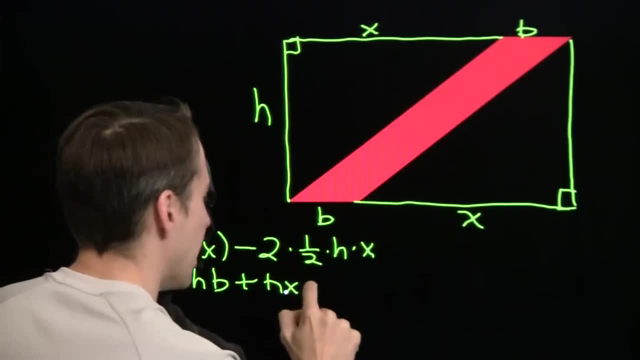 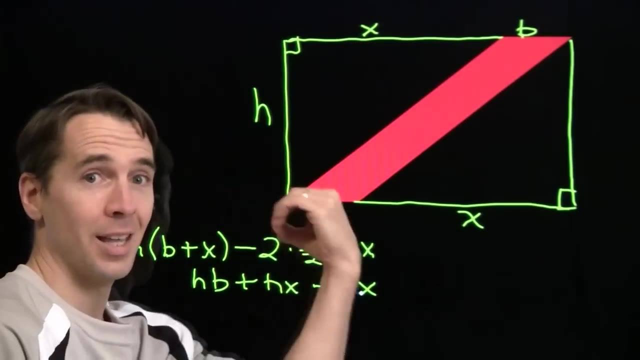 h times b is hb. h times x is hx. 2 times 1 half, and that's just 1, times h. times x minus h times x. Sure enough: hx minus hx, that's just 0.. And we're left with h times. 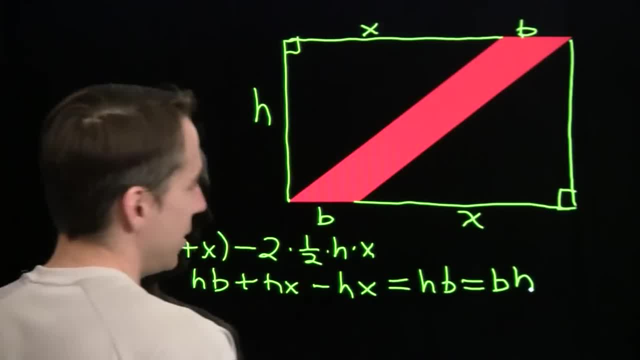 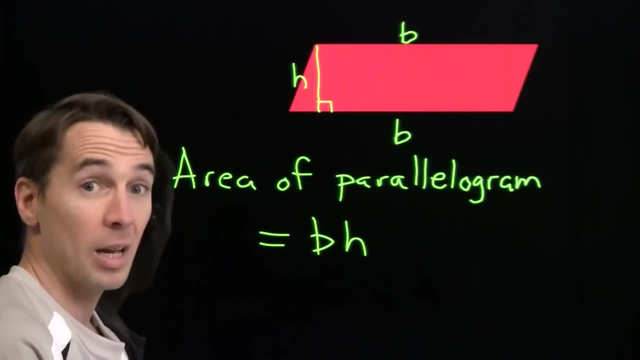 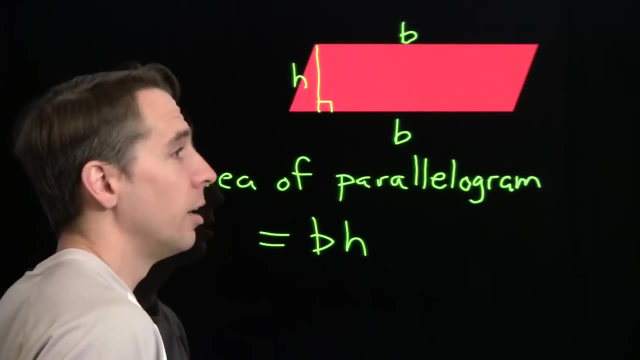 b, which is, of course, the same thing as the base times the height. So this parallelogram base times height. This parallelogram base times height. No matter how you do it, you've got base times height. It's pretty awesome, Harvey, right there. Yeah, all right, What's that Animation? 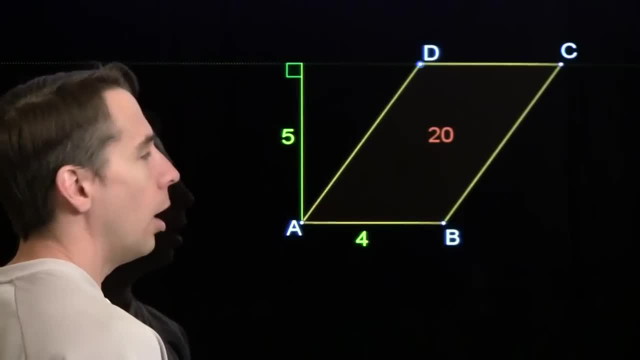 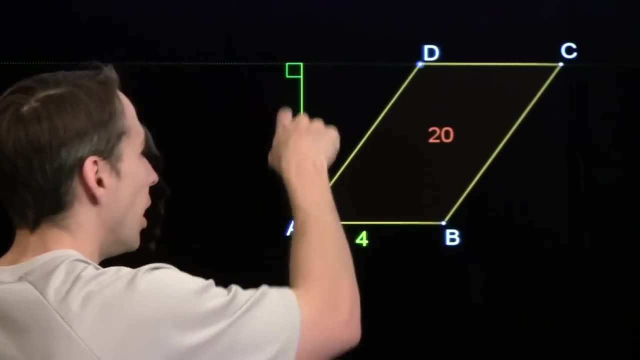 Oh, there is another one. Oh, that's nice. Check this out. Harvey made this for us. Parallelogram Base is 4.. Height is 5. Area is 20.. Let's see what happens when we slide this around.